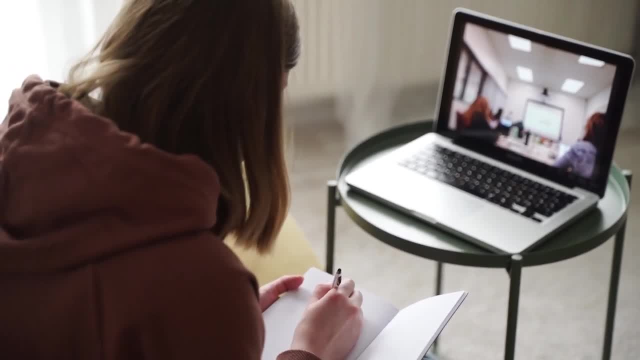 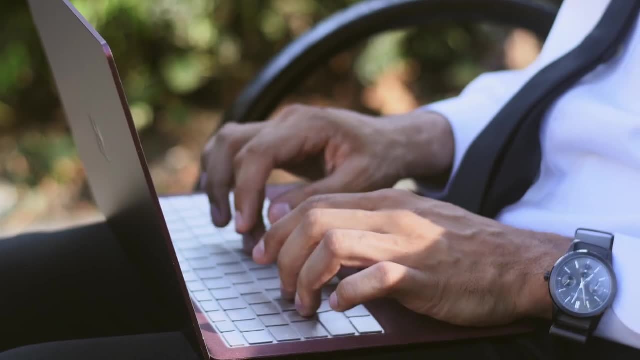 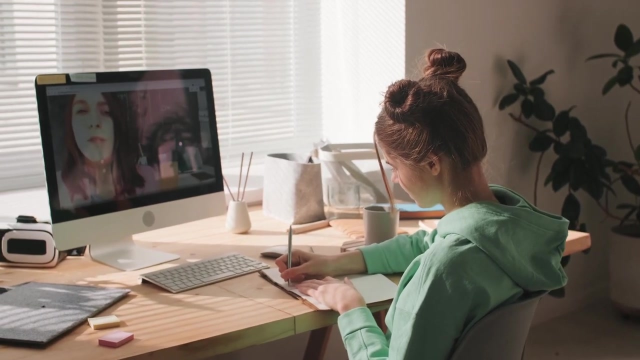 that were adopted a few decades back. Technology has brought about various changes in the way education is delivered and received. From self-learning to flipped classroom approach, we have seen technology make a considerable impact. 5 New Trends in Educational Technology. Here are the top 5 educational technology trends that we are going to see in 2021, and so on. 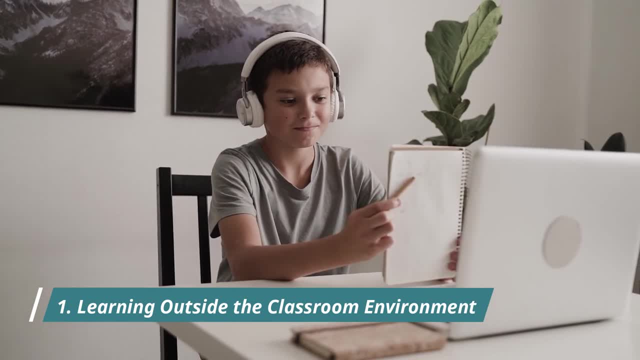 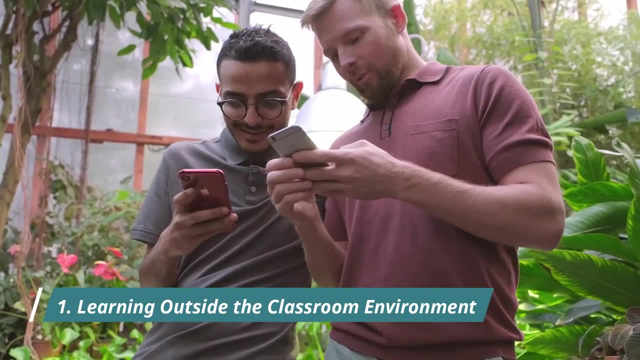 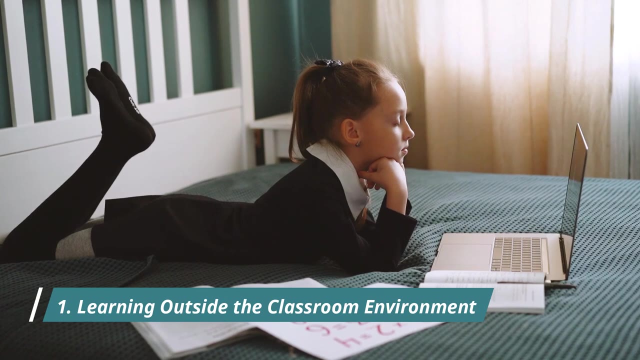 1. Learning Outside the Classroom Environment. Mobile-based devices have taken learning outside of the classroom. With mLearning and eLearning growing in popularity, students can learn at their own pace and time. This trend is expected to keep up, as it is a convenient method of delivering as well as receiving the 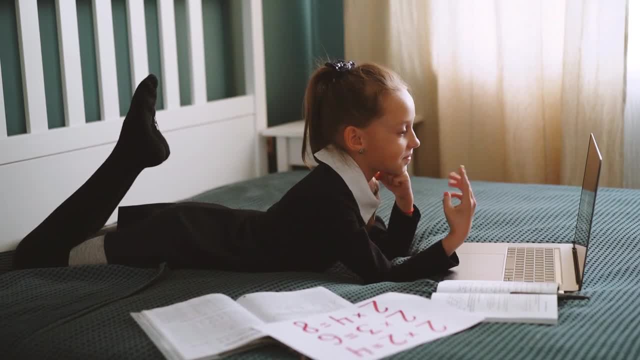 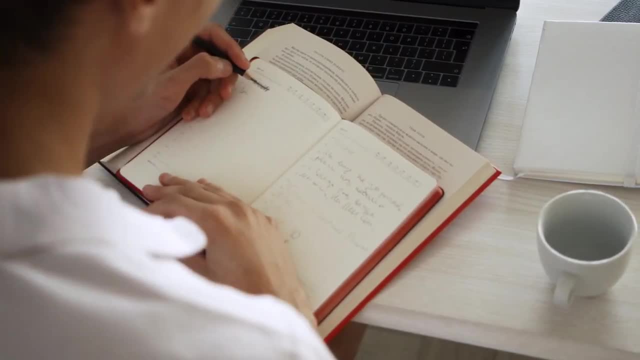 best education. 2. Designing mobile-first, responsive content helps students to go through their courses anytime and anywhere. 3. Internet connection is no longer an issue. with offline reading capabilities, Ebooks can be embedded with many features to enhance the learning experience. 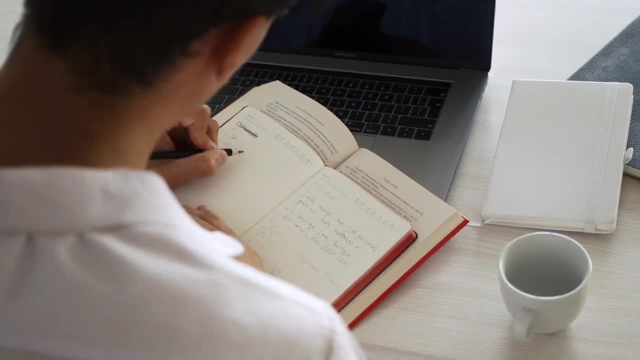 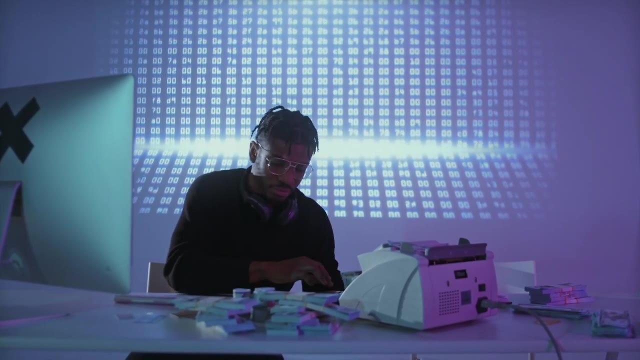 4. Complete with annotation tools, bookmarks, hyperlinks, dictionary search feature. an ebook makes learning more flexible. 5. Most of the educational institutes today have adopted mobile learning into their learning ecosystem. 6. E-learning has become more flexible. Most of the educational institutes today have adopted mobile learning into their learning ecosystem. 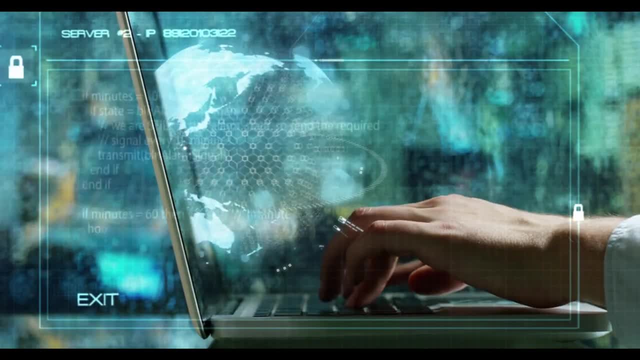 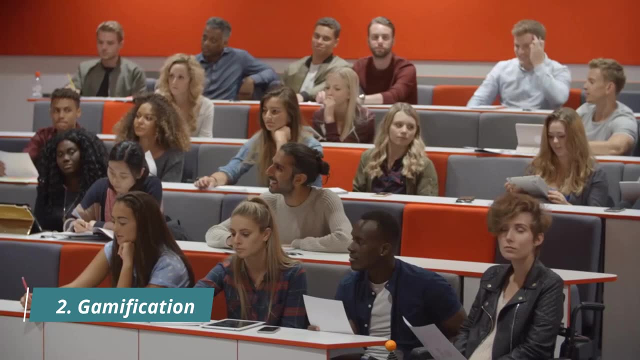 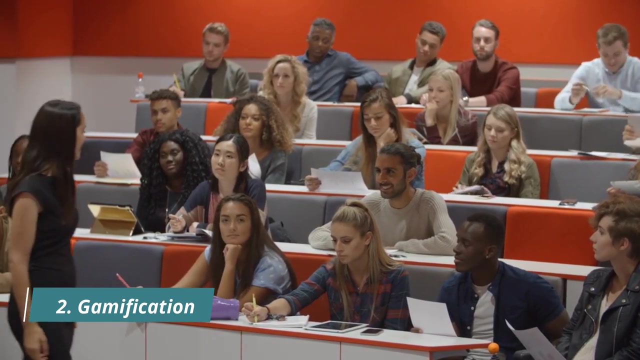 benefiting students and teachers alike. 2. Gamification: Gamification is one of the most innovative trends in educational technology. It has become an increasingly essential part of education in the last few years. The gamification approach uses different strategies, varied activities, badges. 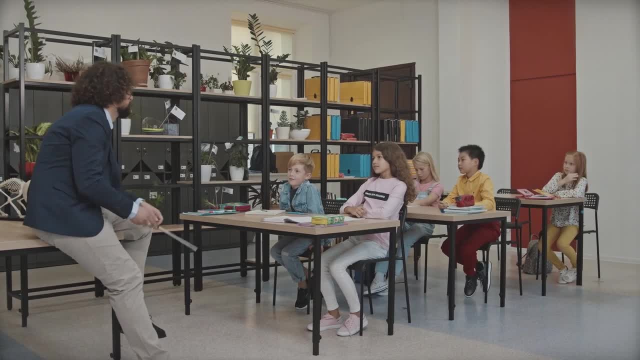 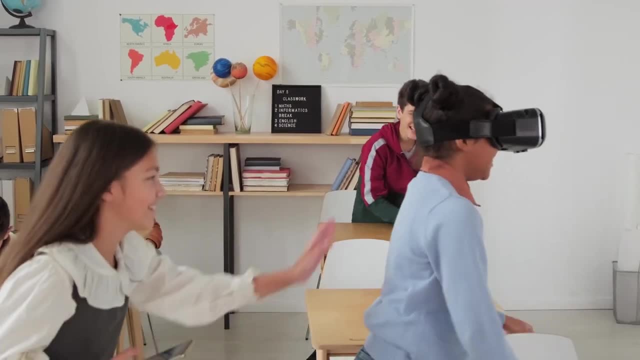 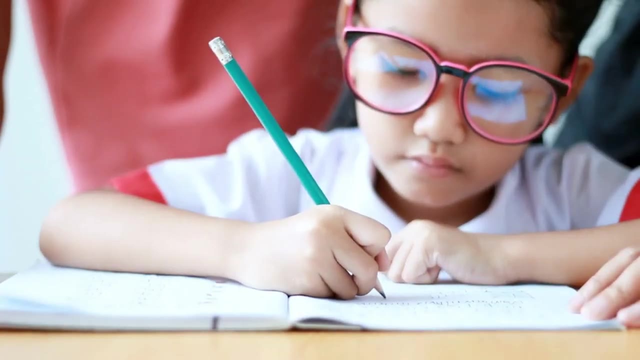 and rewards to promote student or learner engagement. The approach makes use of the various elements and characteristics of gaming culture in designing the courses. It helps the students to become active and motivated learners. Learners play educational games to learn various academic skills and earn points or rewards for completing the assigned tasks. They compete with peers towards. 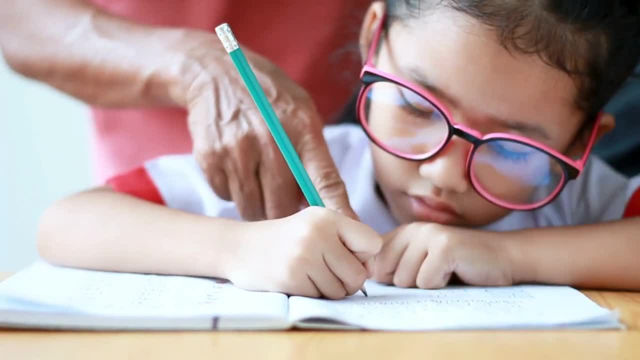 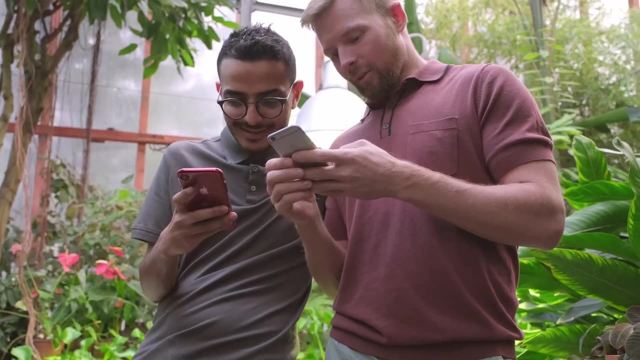 specific objectives or goals. The challenges and rewards help the learners to remain motivated in the process of learning. The game-based approach helps to make the content more fun and interesting for learners. It also makes them aware that gaming and social media are different. Earning badges, coins, rewards. 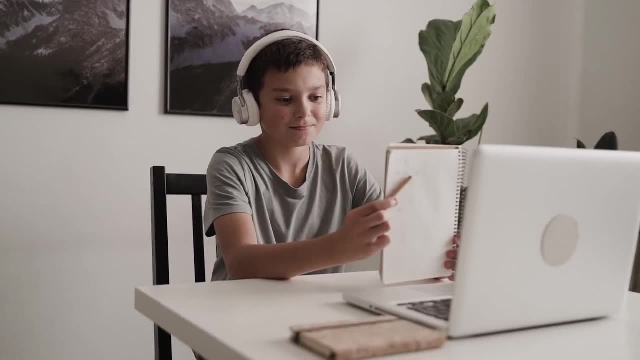 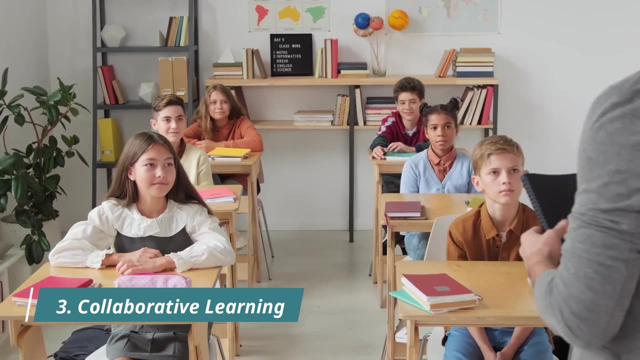 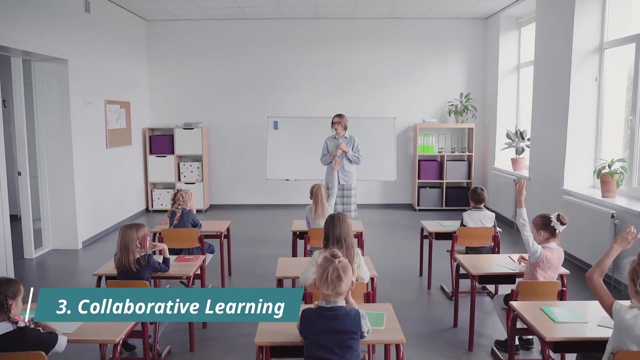 and so more makes the learners pay more attention to what is being taught to them. 3. Collaborative Learning Technology has made it possible for everyone to stay connected. We connect, discuss and enact upon situations collaboratively. This collaborative approach has gained importance in the learning process as well. 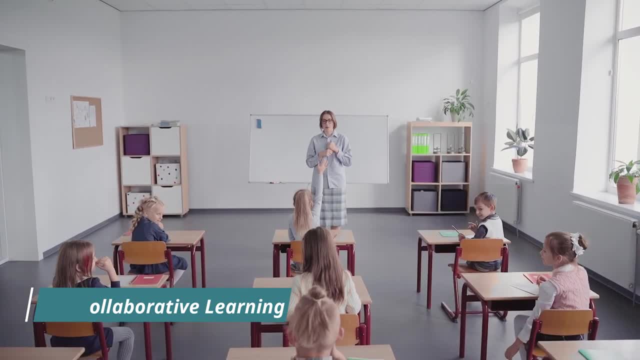 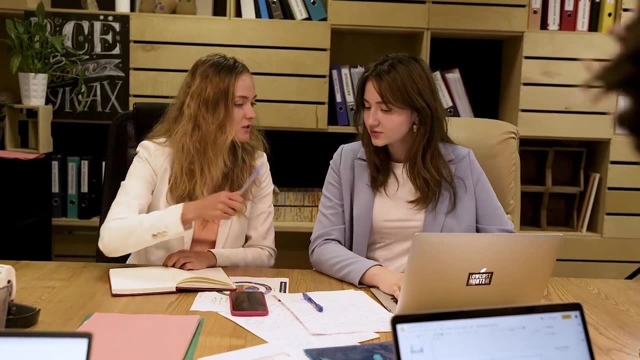 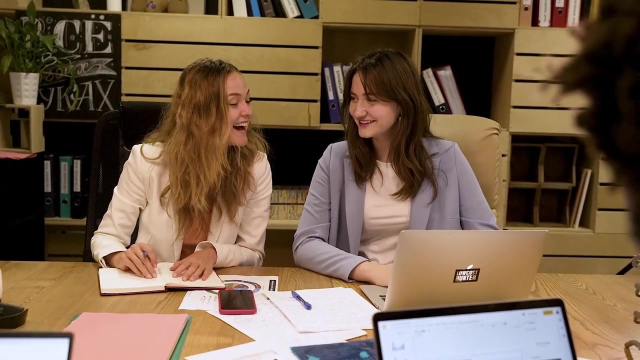 In a classroom learning model, teachers encourage collaboration by assigning group activities and tasks. When students team up together to work on a project or solve a problem, it builds their collaborative skills. Working together improves their understanding and increases engagement. Although e-learning is quite popular, it includes collaboration with features to share and discuss. 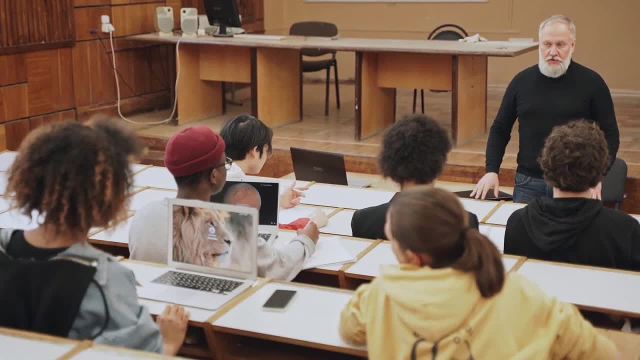 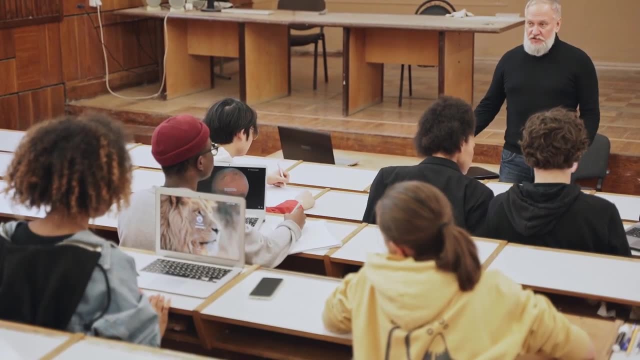 In a traditional teaching model, a teacher enters a classroom, speaks for about 30 minutes and leaves when the bell rings. But today, technology has bridged the gap between teachers and students. You would find teachers and students interacting with each other more often. 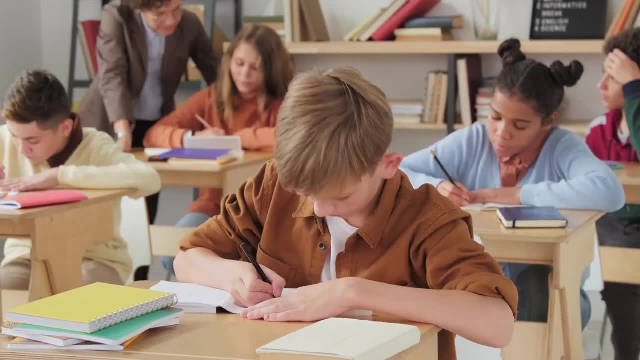 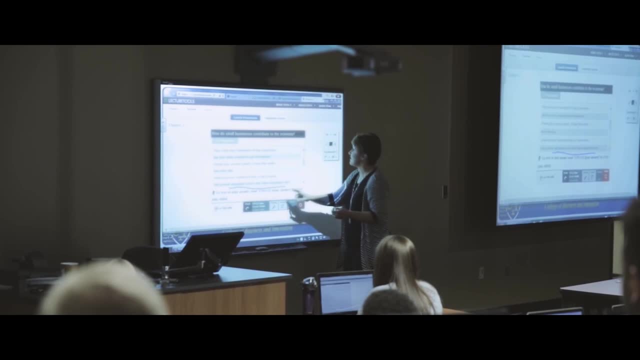 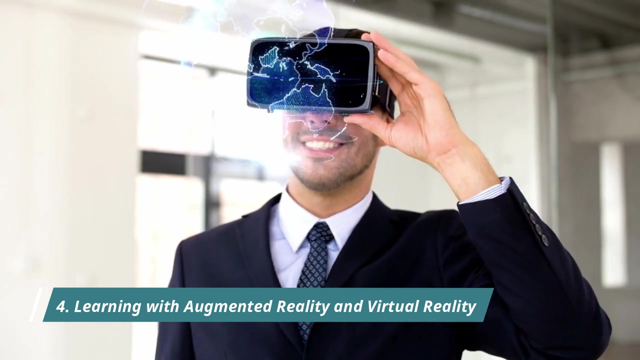 Teachers are far more accessible now and act as mentors to help students in their overall development. This collaborative learning approach helps students to interact with their peers and build their interpersonal skills. 4. Immersive learning with augmented reality and virtual reality. With the introduction of augmented reality and virtual reality into the education, 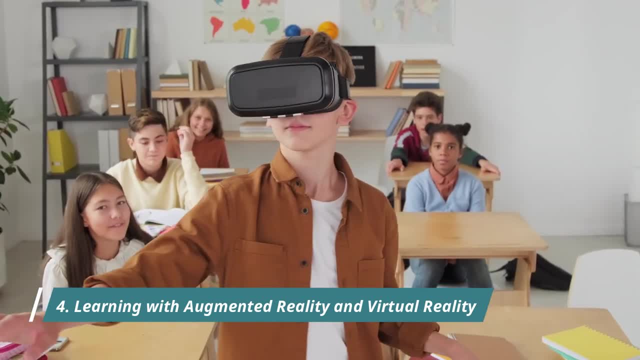 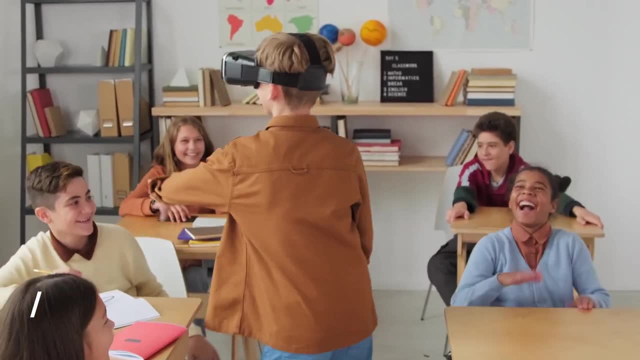 system, it is possible to develop a more inclusive and interactive learning experience system. the classroom learning experience has undergone a tremendous change. learning has become much more immersive than traditional methods. unlike plain images and hands-on experiments in the lab, students can now view enhanced versions of the image and objects on their mobile devices. 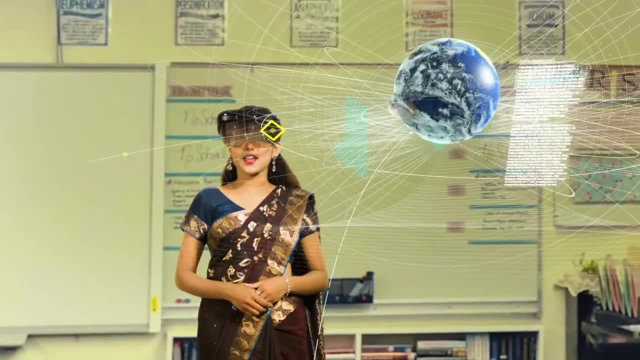 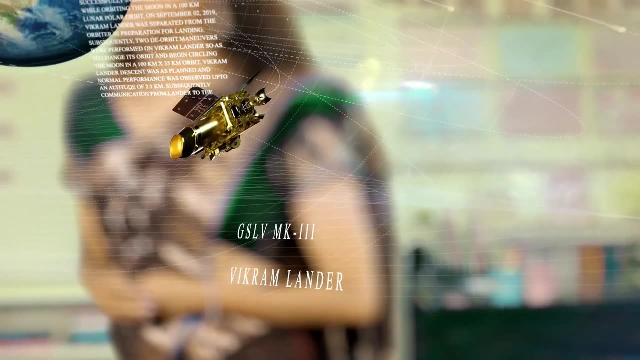 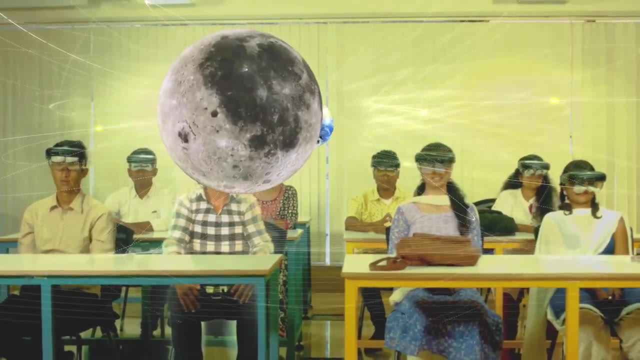 the augmented and virtual reality trends in education technology are making learning a compelling experience. while augmented reality provides an enhanced view of a real image, virtual reality gives a false perception of reality around them. both these techniques have taken digital learning to new dimensions. augmented reality and virtual reality are increasingly being 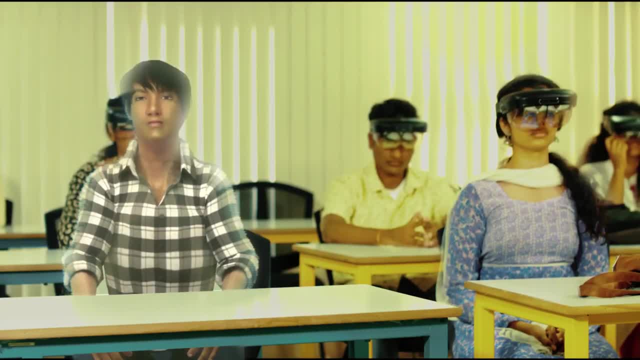 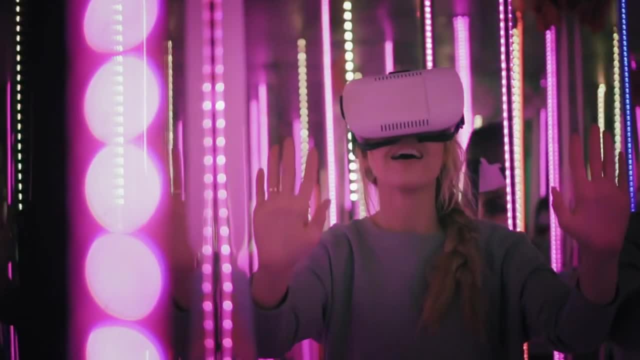 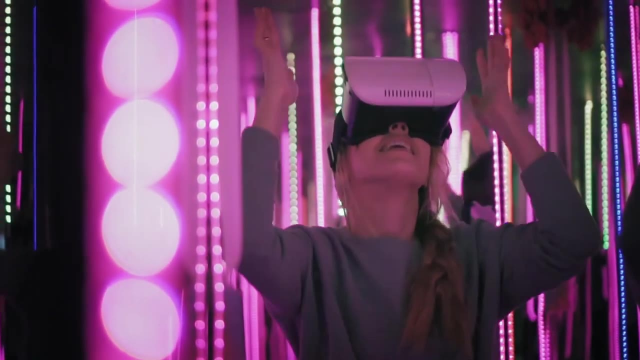 used to explain complex concepts from atoms to planets and from egypt to the coliseum. students can explore and learn so much more. according to edweek's market brief, by 2021, over 15 percent of schools in the united states will have a set of virtual reality classroom kits.